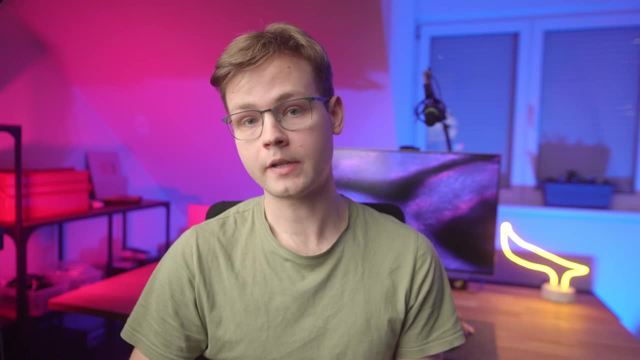 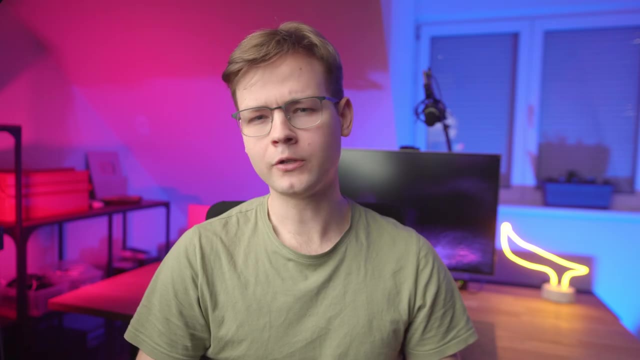 you'll also need to sync your website sources between these two machines and make sure that both machines have the static website generator of your choice installed on them, as well as all the dependencies. Oh, and don't forget the ssh key for deployment. 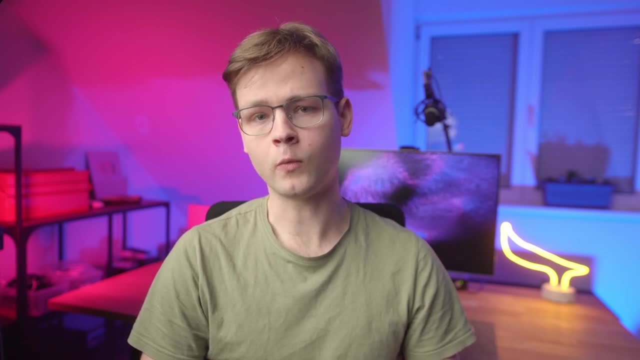 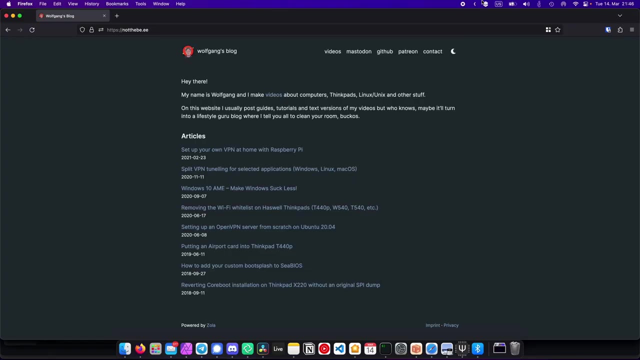 However, there is a different way, and today I want to show you a way to automatically build and deploy your website every time you update it, using github actions. I have a very simple static website over at notthebeatee with a very large backlog of frequently updated articles. 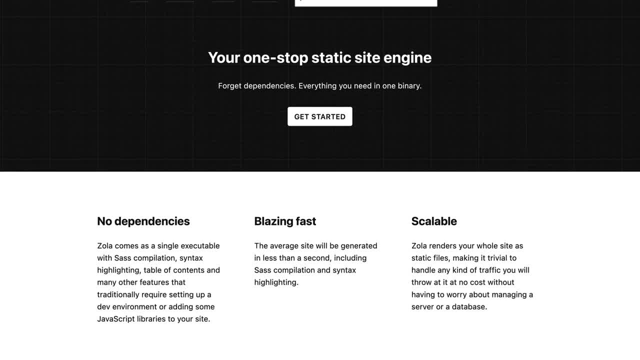 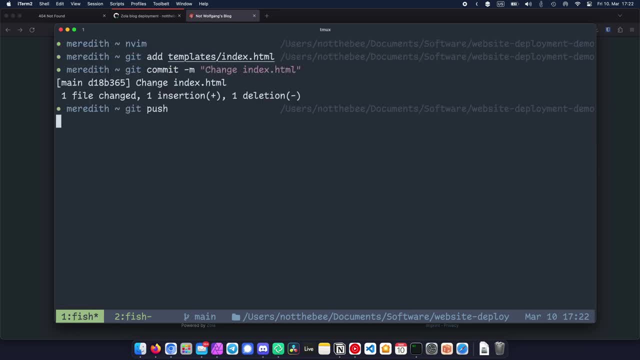 It currently runs on Zola, which is a super simple static site generator written in Rust. The way it works is I have a github repository with the website and then, once I write my bi-annual article and do a git push, the changes get picked up by github actions. 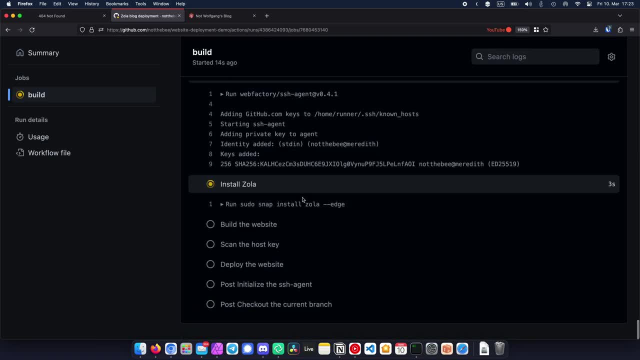 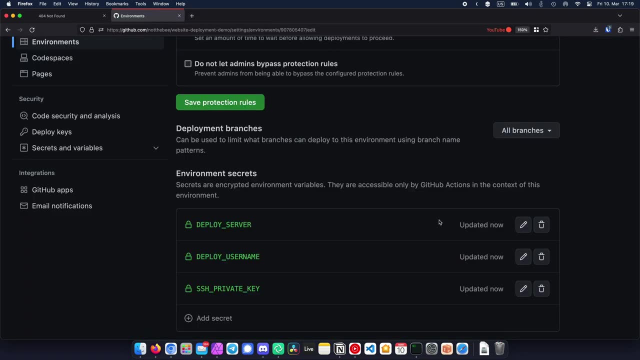 The little magic elves inside the github data center set up an ephemeral linux environment that will clone my repository, generate the static website and deploy it to the server. The ssh key and other sensitive data is stored in the environment secrets, so I don't have to worry about copying them between all of my different machines. 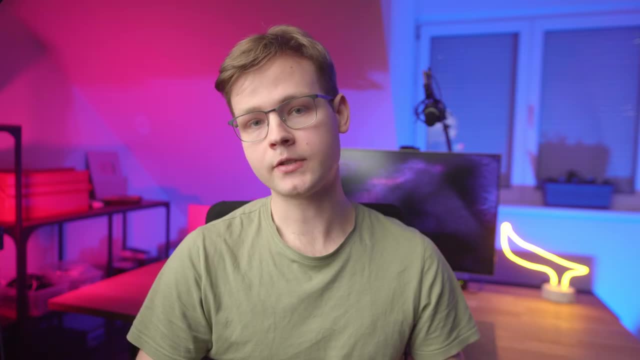 or different linux installations. if you're an avid distro hopper, Now obviously I prefer something more local, so that you don't have to rely on github or any other big tech services, Maybe something like a makefile or simply logging into the server and running git. 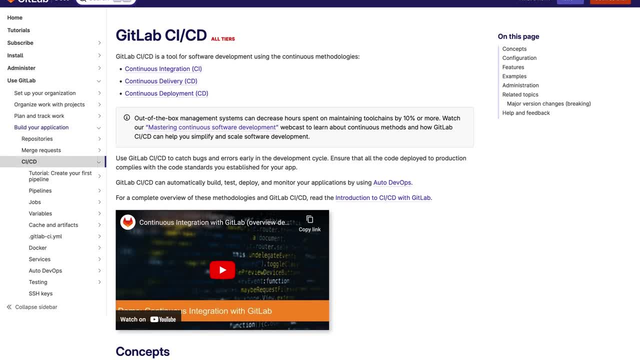 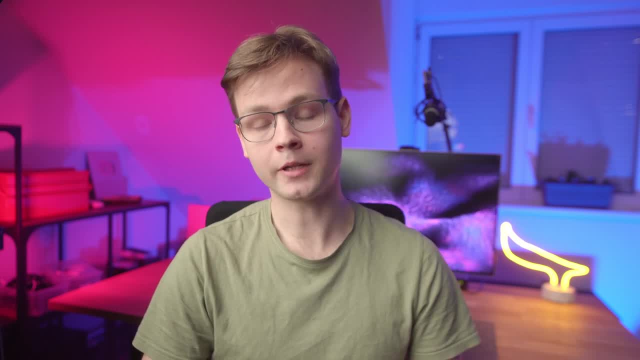 pool every time you push the repository. Plus, if you have a self-hosted gitlab instance, you can do something similar with gitlab-ci. However, in this video, I will only be covering github. So yeah, let's get cooking. 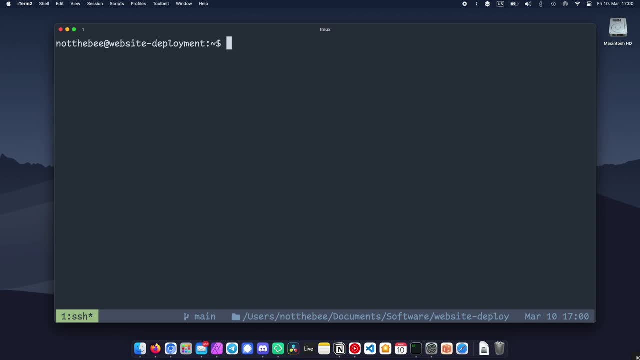 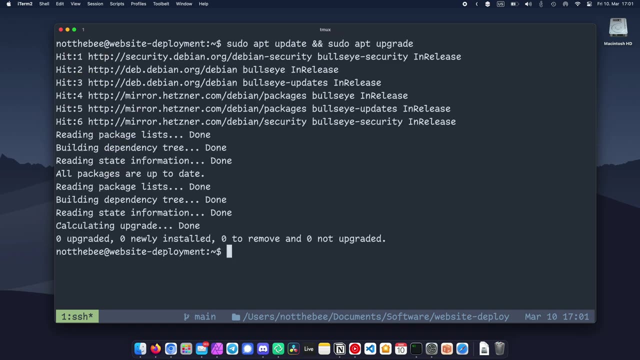 First things first, we need to install Nginx, Certbot and the Nginx plugin for Certbot. I'm on Debian 11, so I'm just gonna type sudo update- double ampersand- sudo upgrade first, And then I'll type sudo apt: install nginx certbot- python3-certbot-nginx. 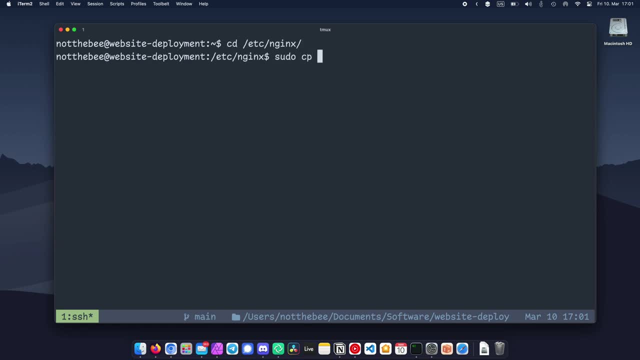 Then we need to go to slash etc. slash nginx and copy the default server configuration from sites available into conf, dot d, slash static dot conf. Now let's edit that file, and here we want to remove everything apart from this last block. Then we're gonna uncomment everything and change a couple of parameters. 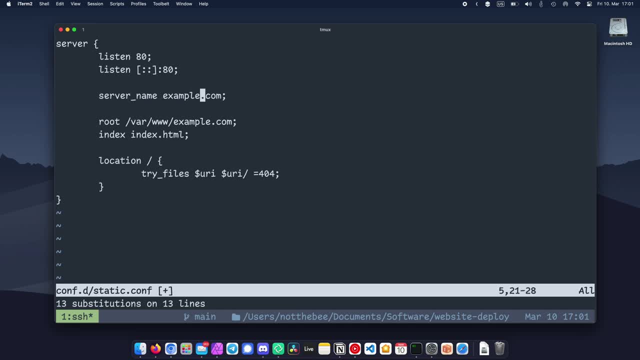 Server name. here you're gonna want to put the address of your website, in my case not the b. you should also make sure that the domain name you're using is already pointing to the ip address of your server, And root is gonna be the folder which will. 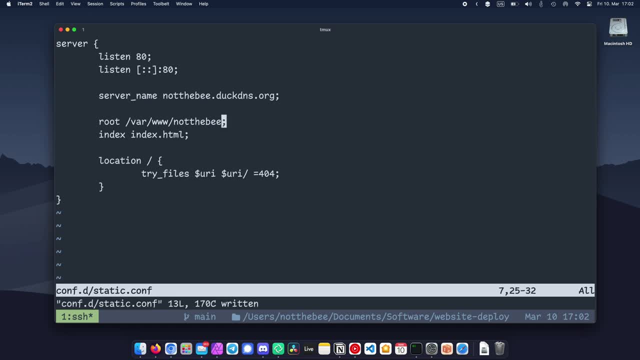 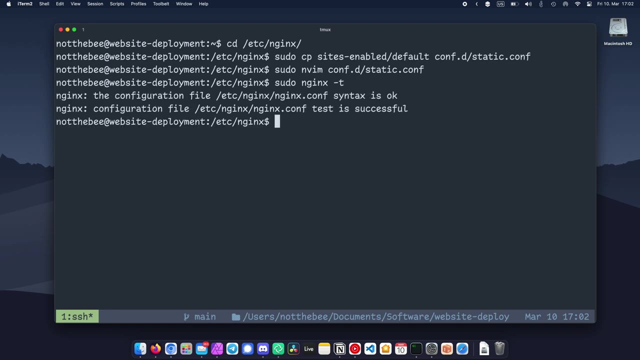 contain your static website. I'll go with slash, var, slash, www slash, not the b, and you can obviously choose any directory name that you like. Just make sure to replace this path in all of the commands and the configuration files. Once that's done, you can close the file and type sudo nginx, dash t to test the configuration. 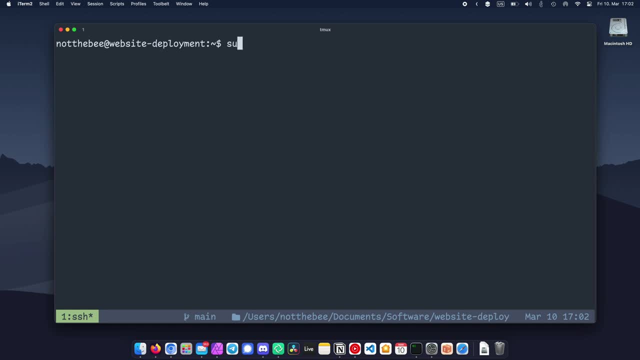 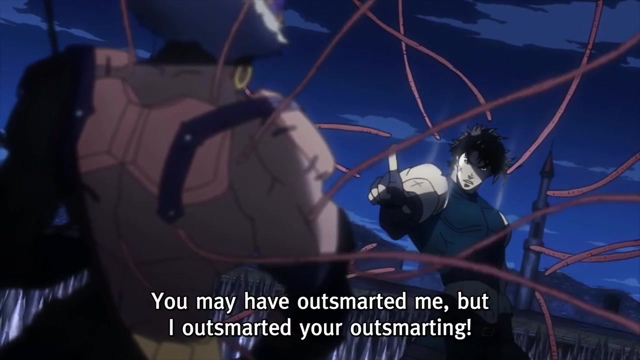 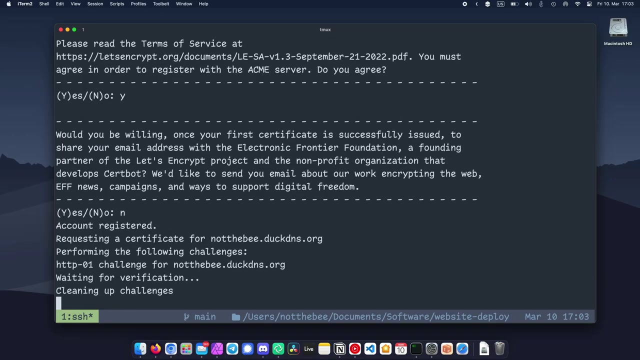 Finally, we're going to generate the ssl certificates for our new website, For the. For that, let's type sudo, certbot-engines-d and the domain name of the website. Here you're gonna want to put your email. As you can see, I tried to get away with root at localhost, but it has outsmarted, my outsmarting. 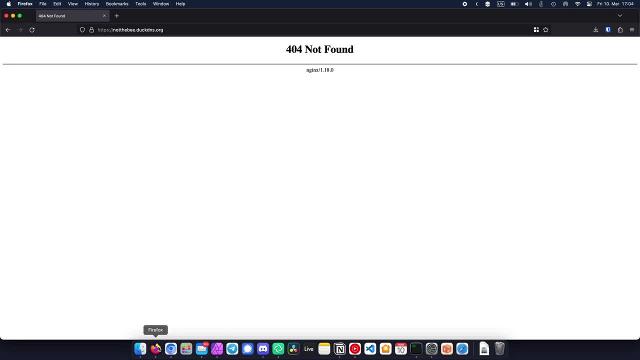 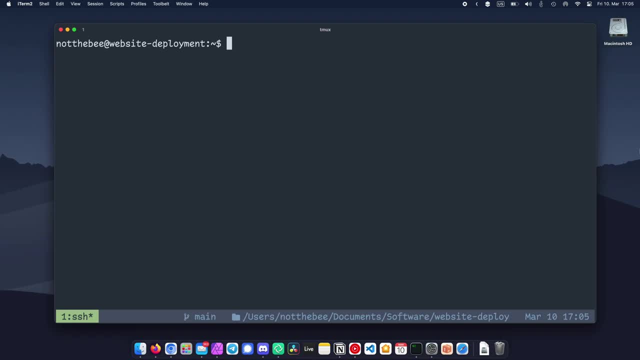 Now let's open our website in the browser and 404.. That's exactly what we want to see. since our website directory doesn't actually exist yet, Now we need to create a separate, unprivileged user that we'll only be using to copy our 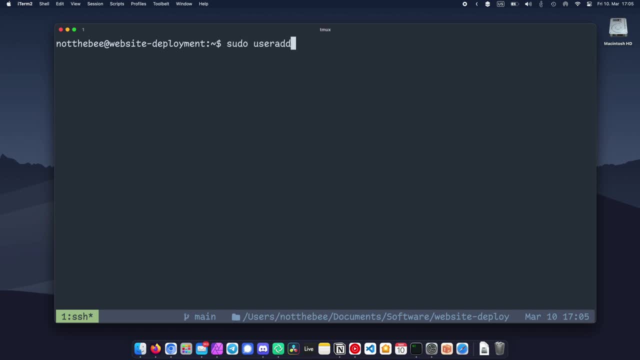 website over to the server. Let's type: sudo useradd-G- www slash data. if you're on Debian-based distro or engines. if you're on a Red Hat-based one, deploy-m-d slash- var slash- www slash, not the p. Now we'll create our ssh keys, so let's switch to our local machine and type ssh-keygen-t. 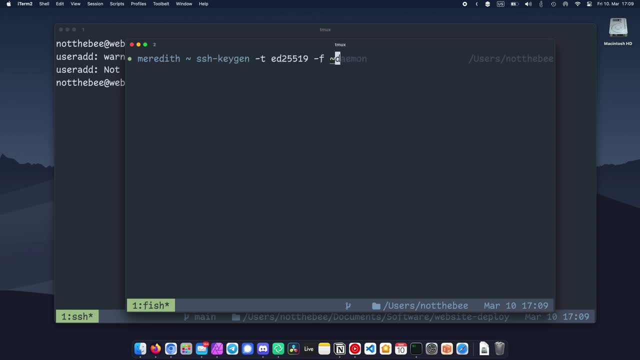 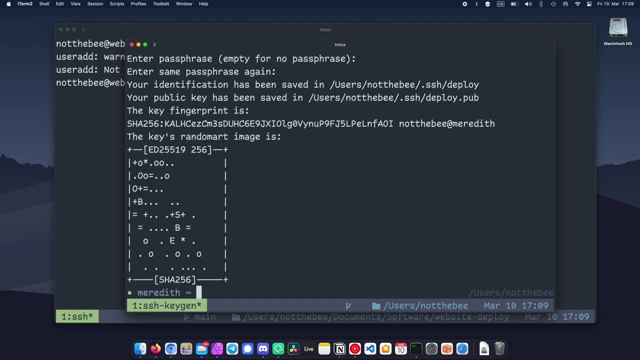 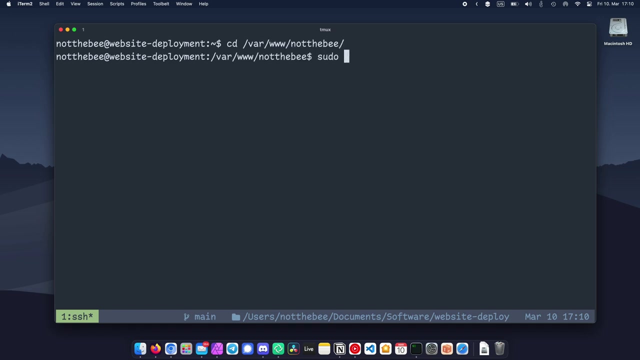 ed25519-f: tilde slash dot. ssh, slash deploy. We'll also set an empty password here by pressing enter twice when asked for one. After that, we're going to create an ssh folder in our new user's home folder. slash, var, slash, www slash, not the b. 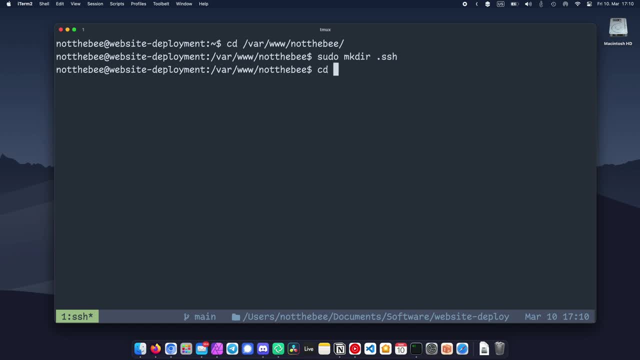 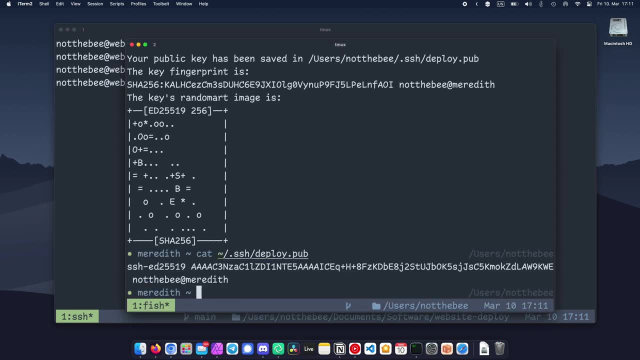 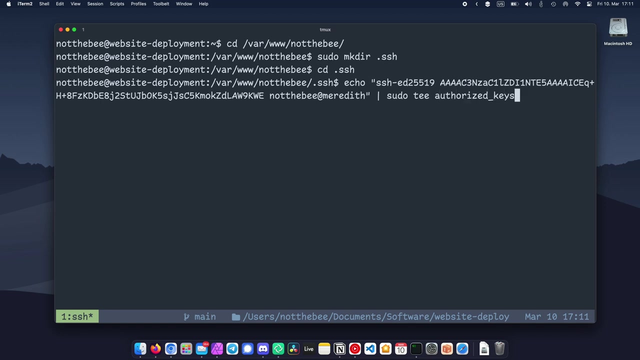 You'll have to use sudo for that. Once that's done, we're gonna cd into the folder and put our public ssh key that we just generated into a file called authorized underscore keys, like so. Finally, we need to make sure that the ssh folder and our authorized underscore keys 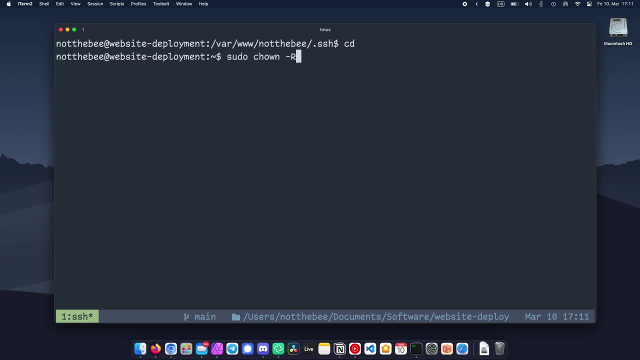 file belong to the deploy user, so let's type the following commands: sudo chown-R- deploy colon www. dash data or engines. slash- var slash- www slash, not the b. sudo chmod 700: slash var slash- www slash, not the b. That's it. 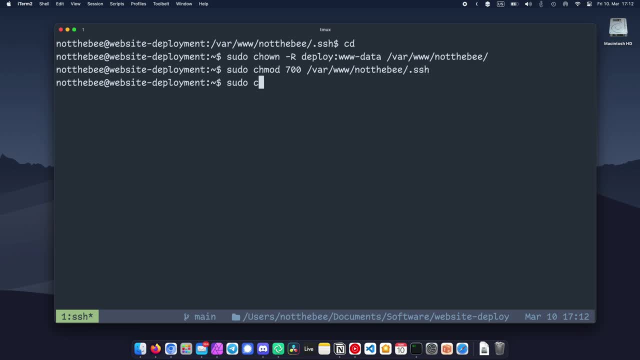 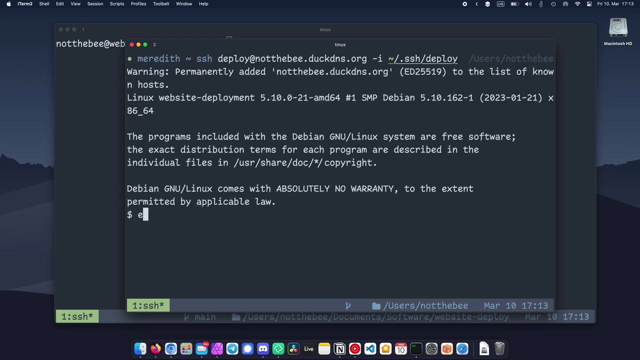 We can now test our setup by switching to our local machine and typing ssh deploy at server ip: dash i tilde slash ssh deploy. Now we're actually getting to the meat of this tutorial, and that is deploying our websites. As you can see here, I have a folder with my website files. 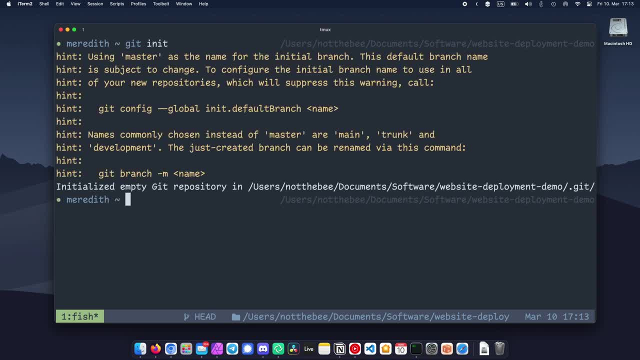 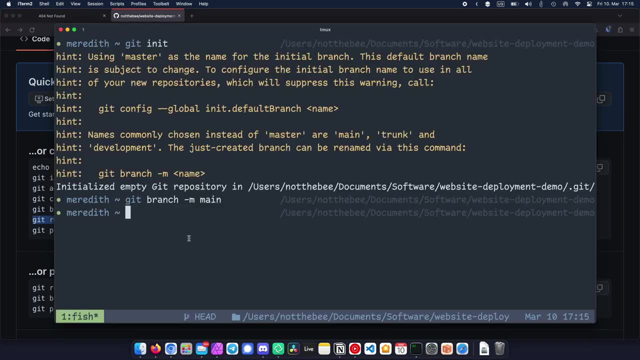 And if you haven't done so yet, you need to initialize a git repository by typing git init and then create a repository in github and add it as the remote origin. Now we're going to create a hidden folder in the root of a repo called github and then 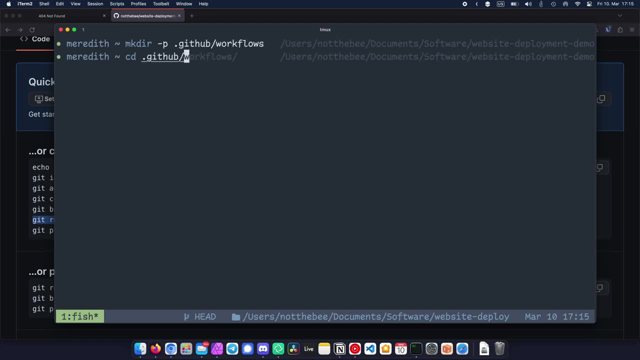 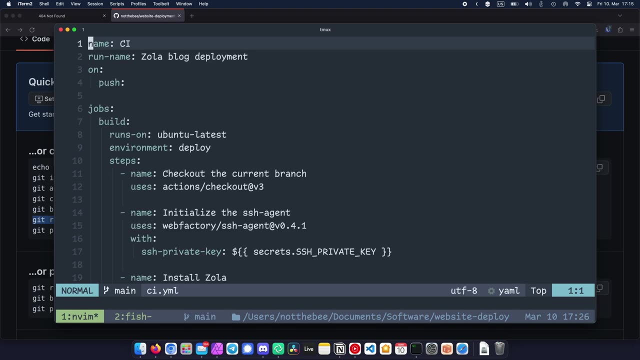 create another folder inside of it called workflows. And finally, we're going to create a file called cuiyml. I wrote a little template, which you can find in the pinned comment of this video, so I'm just going to copy and paste that and let's go through it line by line. 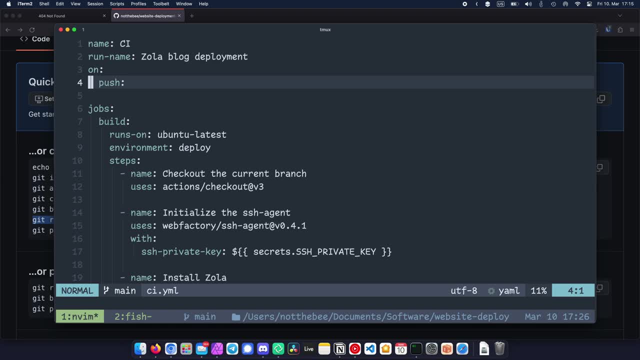 So first, this workflow is going to run. First, this workflow is going to run every time we push to this repository. It's going to run in an Ubuntu VM, which doesn't really matter all that much. It's going to check out the repository. 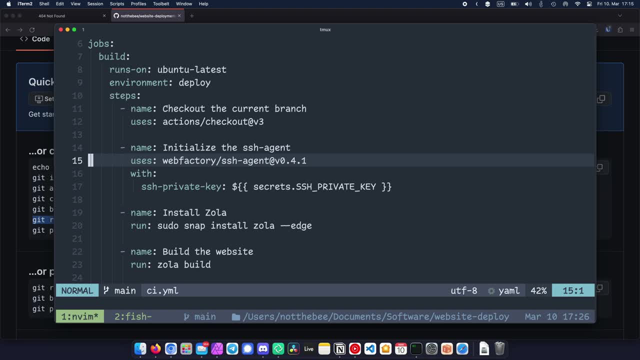 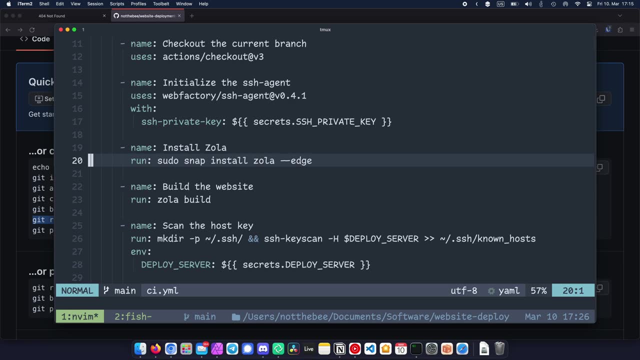 And then it's going to add our private ssh key to the ssh agent- And don't worry, we're going to set up our secrets later. Then it's going to install a static website generator of your choice. For me it's Zola and for you it can be something like Hugo Jekyll or even SSG5.. 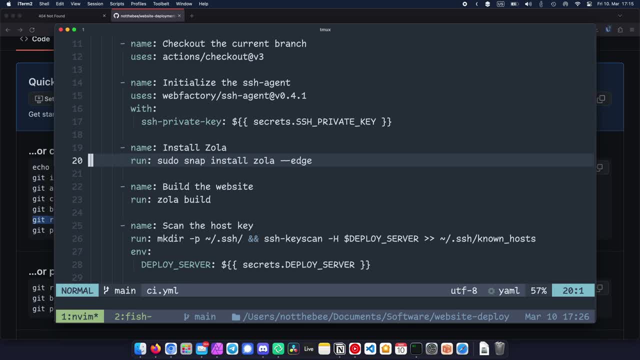 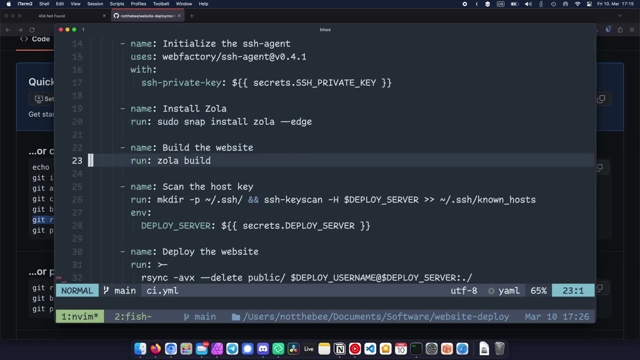 This will run a full-fledged Ubuntu box, so you can basically just sudo, apt, install whatever. I'm using snap here, because Zola is not available in Ubuntu. Then it's going to run a build command that will actually generate our static website. 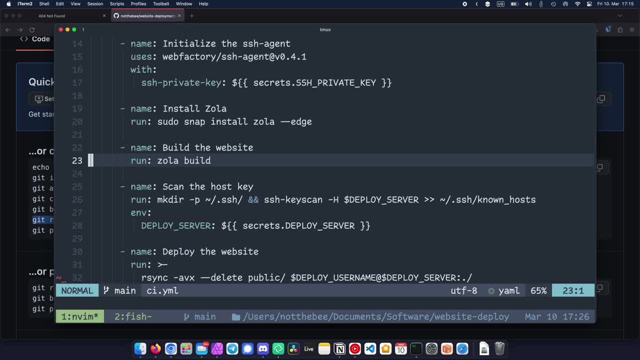 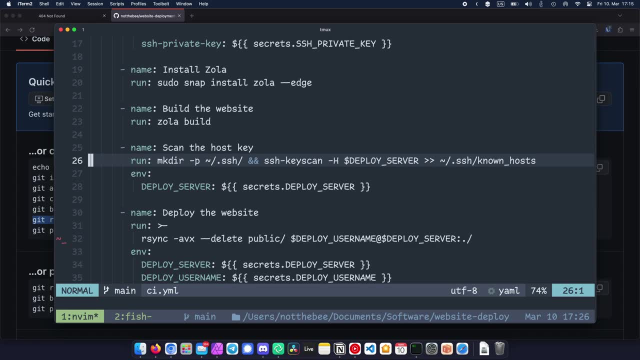 Any command that you will put here will be executed in the root of your git repository. Now we are moving to the process of copying our resulting website to the server. Before doing that, we're going to run ssh keyscan in order to avoid this message that. 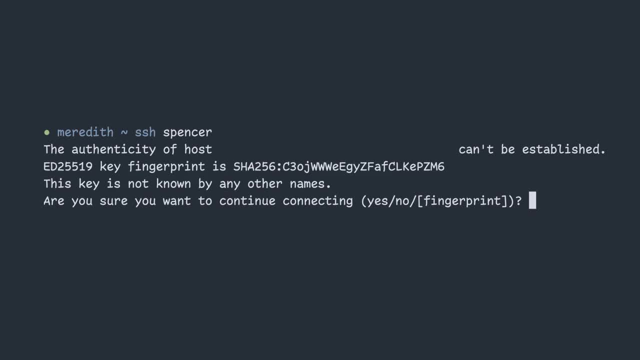 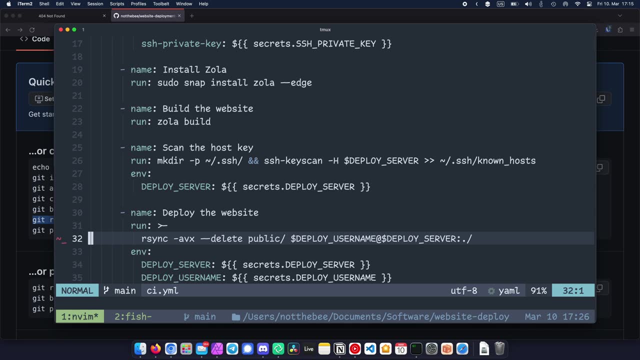 you usually get when you try to log in to an ssh server for the first time, And then, finally, we're going to rsync the public folder with our generated website to the server. In my case, Zola puts the generated website into a folder. 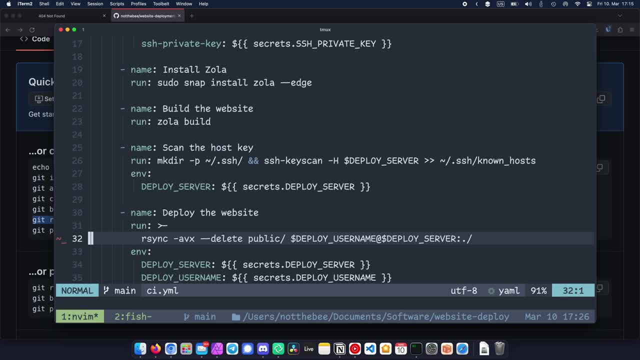 And this will obviously depend on the website generator that you're using. Also, make sure that you have slashes after both source and target folder names, otherwise rsync will just create a new folder inside your target folder and copy the files in it. Once you've changed everything that you wanted to change, you can save the file, but don't. 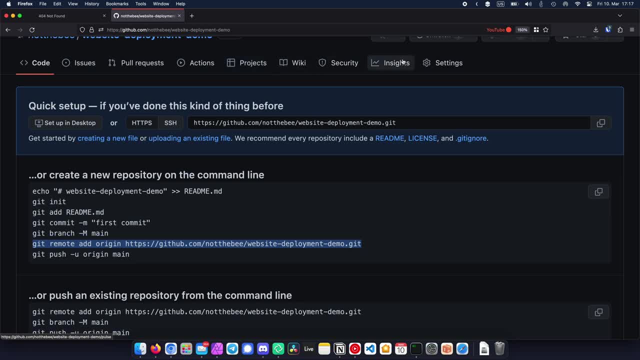 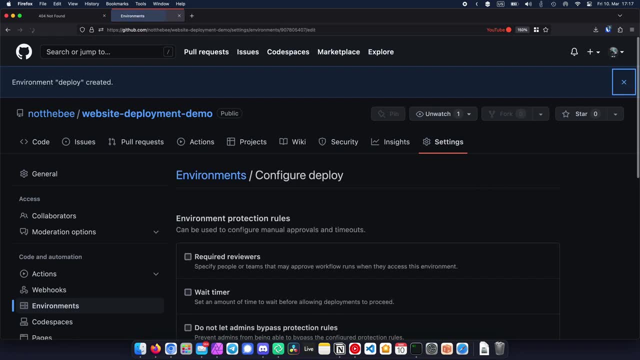 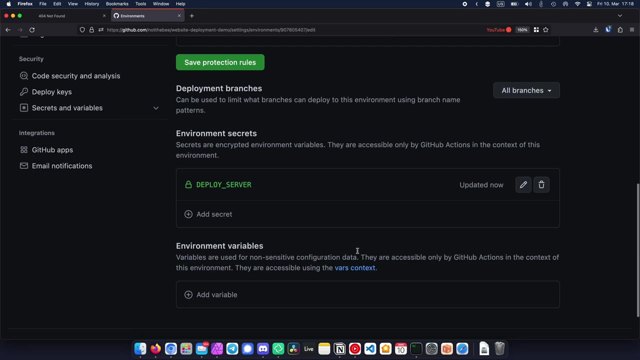 quit the text editor just yet. Before we commit our changes, we need to go to our github repository settings, then click on environments and then create a new environment called deploy. Here we'll need to create three secrets: Deploy underscore server, which will be the IP address of the server that hosts your website. 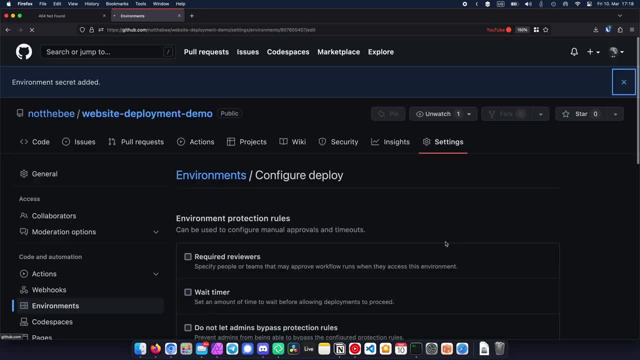 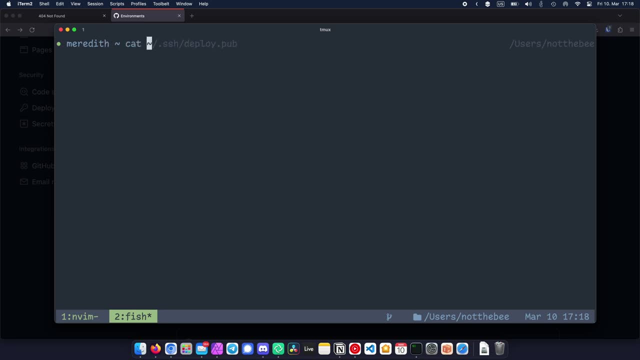 Deploy underscore- username, which will be deploy in our case, And ssh underscore- private underscore key, which is the private key that we generated for our deploy user. You can show the key by typing cat tilde slash dot ssh slash deploy in your terminal, if you're. 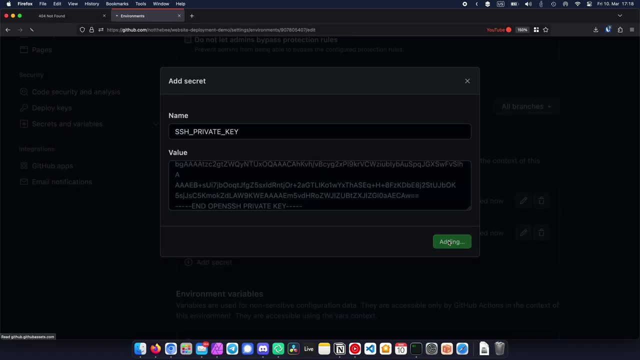 on mac or linux, and if you're on windows, you can simply navigate to the ssh folder in file explorer and open the deploy file with notepad. These variables are not going to be visible to any github user, So we're just going to go ahead and create a new one. 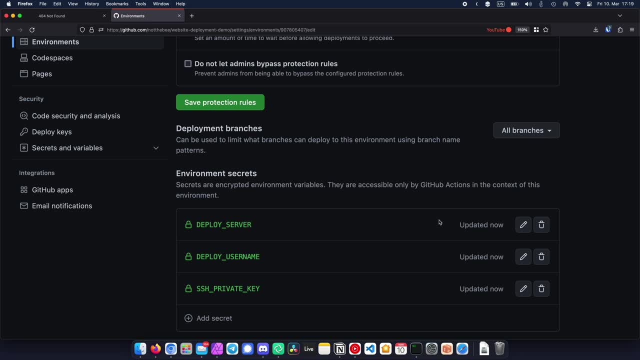 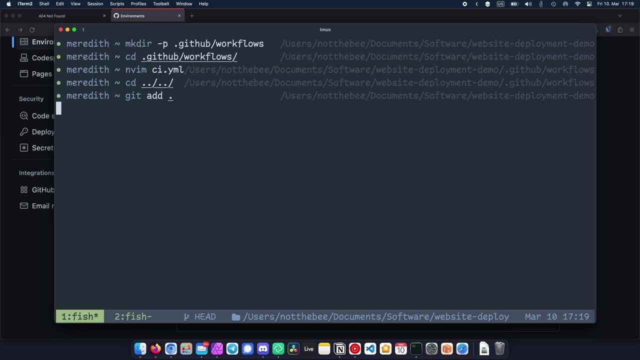 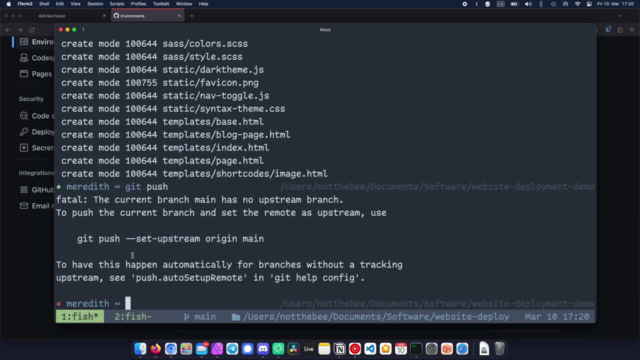 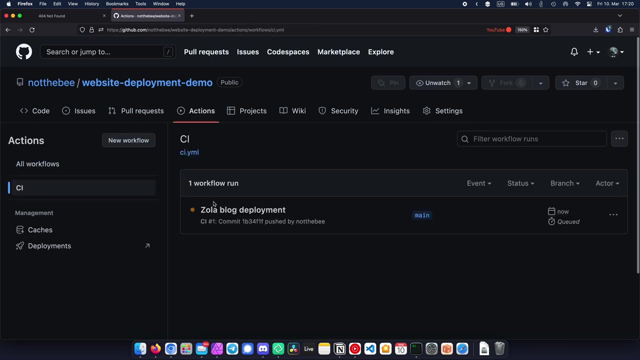 Now we're finally ready to deploy our website, so let's go back to our terminal and type git add dot, git commit, dash m. add github actions, workflow and git push. Now let's go back to our github repository and check on our first deployment. 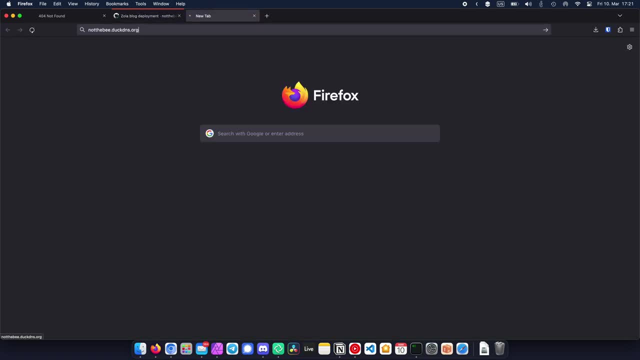 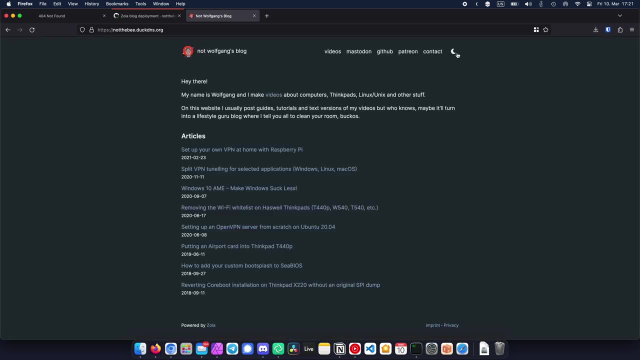 As you can see, it is now done. So let's open our website in the browser, And there you go. Now you can add ci slash cd for web applications to your resume. I mean sure it's a website and not an application, but hey, everything is an app these days. 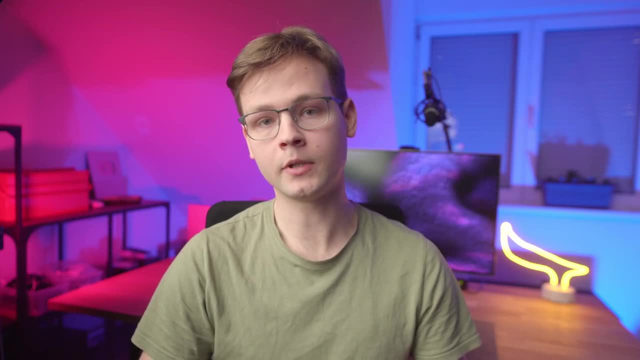 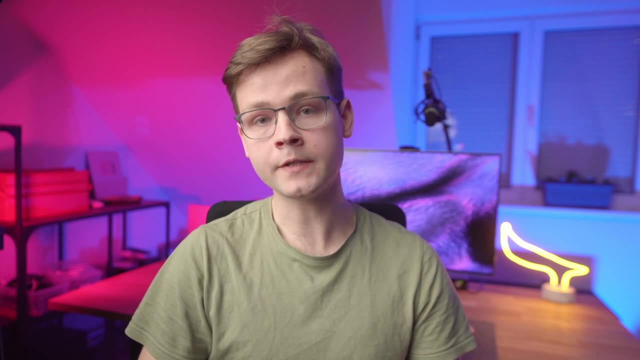 so So there you have it. We learned a super simple and reliable deployment workflow for a static website and I hope you guys enjoyed it. And if all of that sounds a bit too overwhelming and if you still want to create an amazing website or an online store for your business without becoming a command line wizard, you 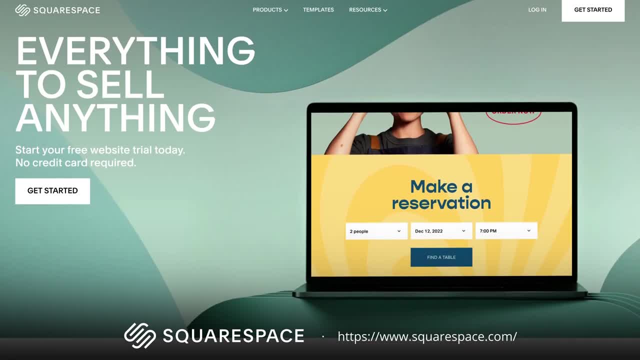 should check out today's sponsor, Squarespace. Squarespace is the perfect solution for you. Squarespace is the perfect solution for you. Squarespace is the perfect solution for you. Squarespace is the perfect solution for anyone looking to create a stunning website.